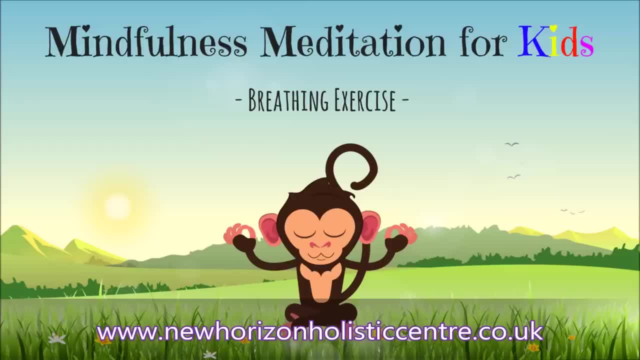 Hello, Focus your mind on your chest rising and falling with each breath. Think of nothing else, just your chest rising and falling as you breathe. You don't have to breathe deeply, just breathe naturally and just focus on how Your chest just rises and falls as you breathe. Notice how your breath flows in and then out. 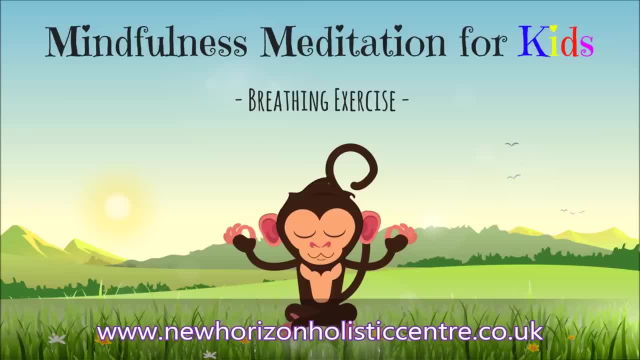 again, Notice how your chest gently rises and falls, because your body knows how much air it needs. So sit quietly seeing in your mind's eye your breath flowing gently in and out of your body. Again, feel your chest rising and falling and when your attention wanders, just bring your focus back. 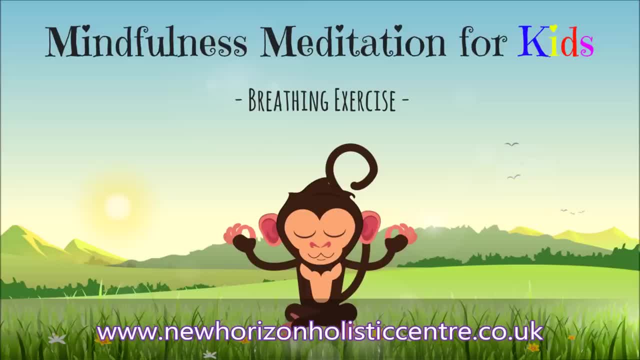 to your breathing. So when you want to think about football or going to school or playing out with your friends, just bring your attention back to your breathing. Feel your chest just rise and fall. That's all you have to think about. Simply let the thoughts pass on by. 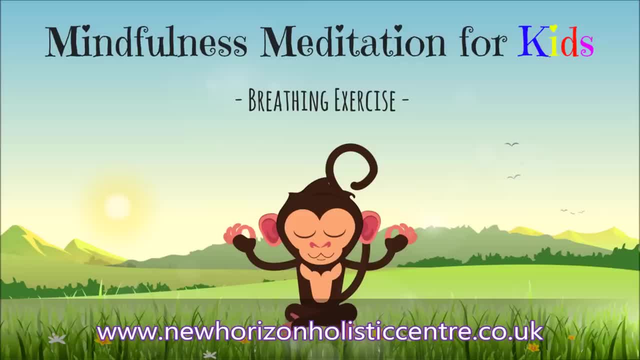 See how your breath continues to flow Deeply, calmly, slowly and gently. You just breathe, Feel the air entering through your nose, Feel the breath flowing through the cavities in your sinuses And then down into your lungs- cool, clean, fresh air flowing gently into your body. 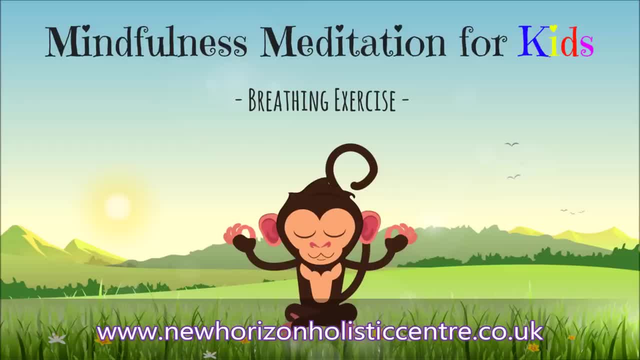 What was that just now? Yourimin killing Recall. Feel the air releasing down into your lungs. Just let all the random thoughts come and go. Do zone individual sounds each minute. wave to them if you want to. How Your phosphate Olha. Watch your assemble shortages. 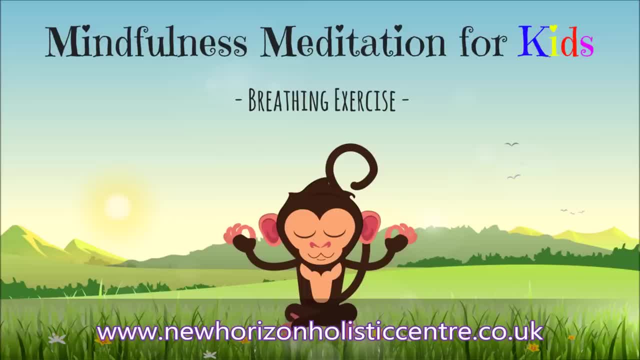 Repeat this naturallylov revoltr. notice them and then return your attention back to your breathing. Feel your breaths, feel each breath, really feel them as you breathe in and then breathe out again. Feel how your body responds to each breath. this is keeping you grounded. 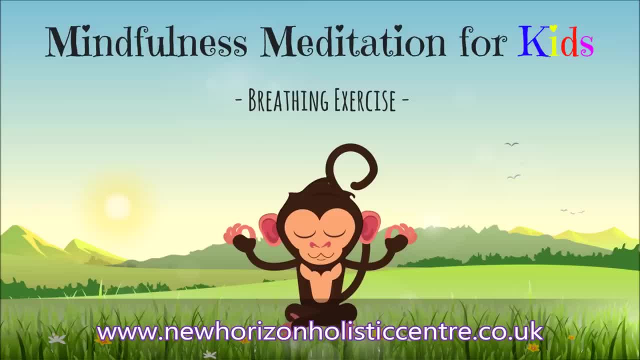 And you can feel how amazing it is just to breathe. You can really feel that this is what is keeping you alive: You are breathing. how amazing just to be able to breathe. Sometimes your mind may wander again, but that is ok, that is not a problem at all. 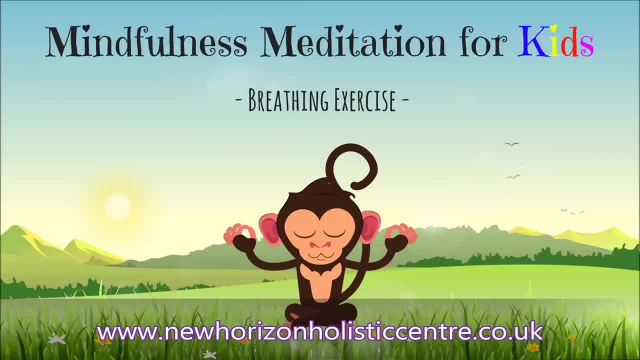 If this is happening to you, just bring your attention back to your breathing Now. bring your focus onto your mouth. With your lips slightly apart, you can feel the breath leaving your body. Can you feel it? Can you feel the breath, that warm air? 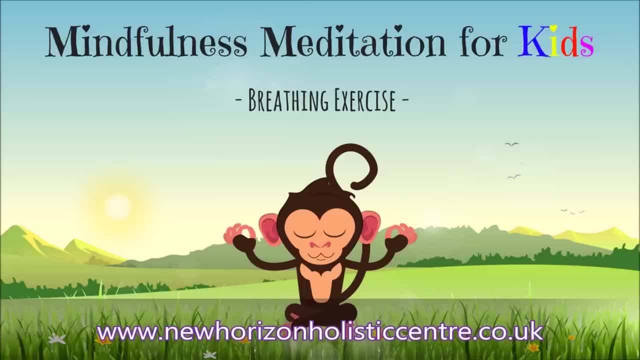 Can you feel it? Can you feel it Leaving your mouth? You can feel how warm your breath is as it passes through your lips And you can feel the vibrations as they leave a tingling sensation on your lips. So focus only on the breath leaving your body. 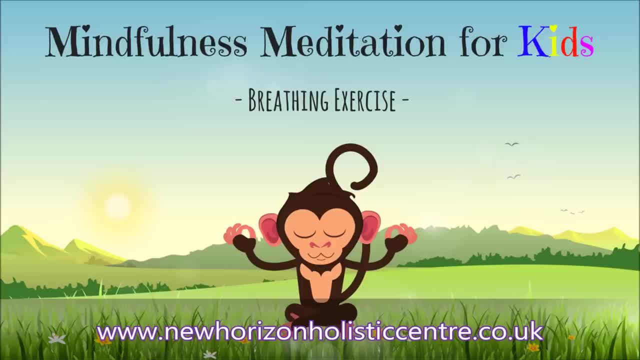 Don't worry about the breathing in, Don't worry about the breathing out. Just focus on the breath coming out of your mouth. Really feel it. Try to be at one with your breath. You are your breath. Just breathe, Just breathe. 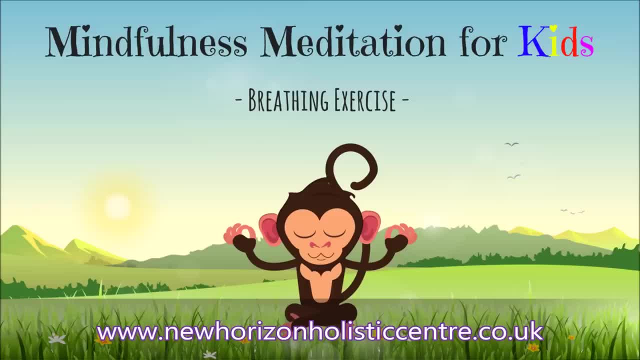 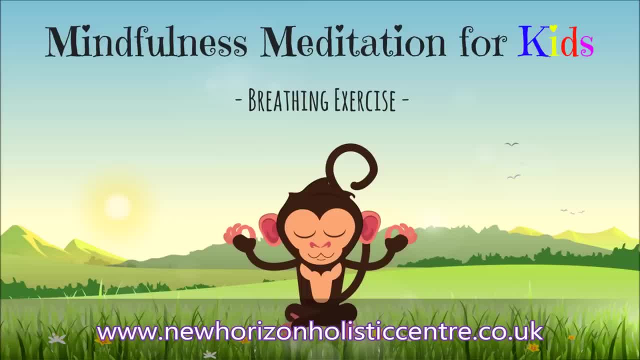 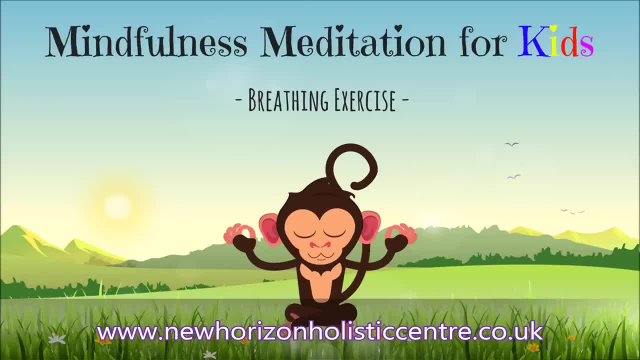 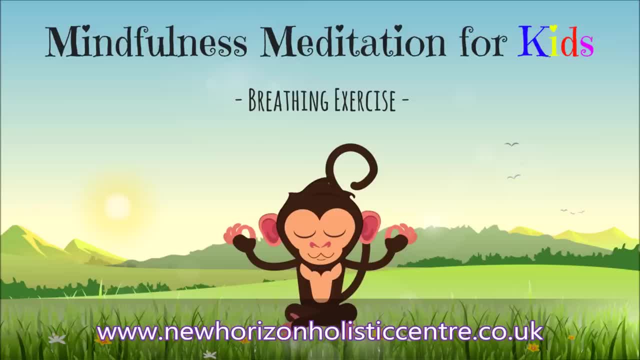 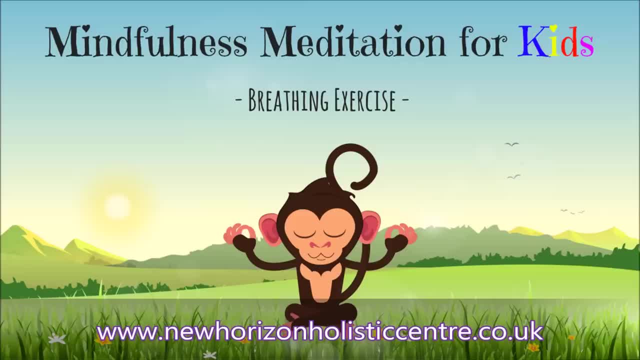 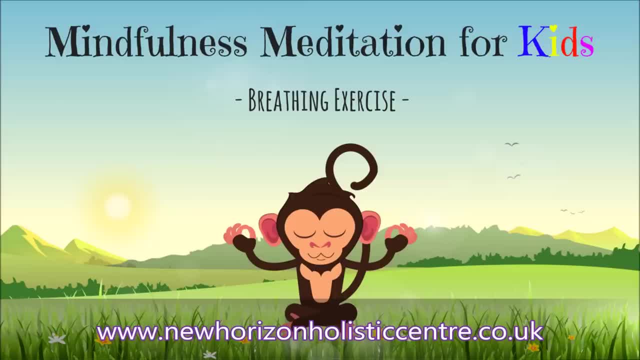 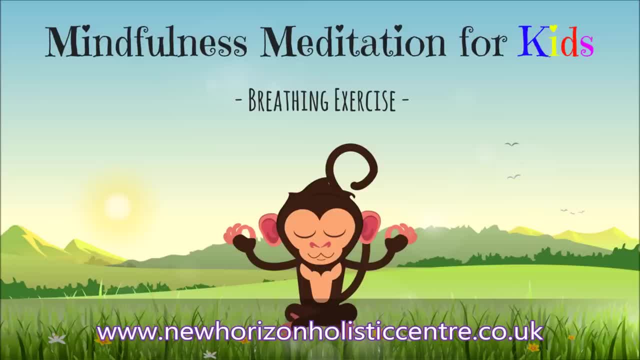 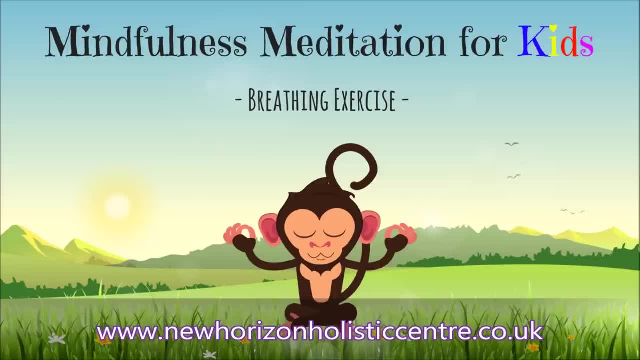 now You feel so peaceful, so safe, so very calm and so very happy. Now it's time to bring your attention back into the room. So take a long, slow, deep breath in and breathe out slowly and gently. Again, deep breath in. 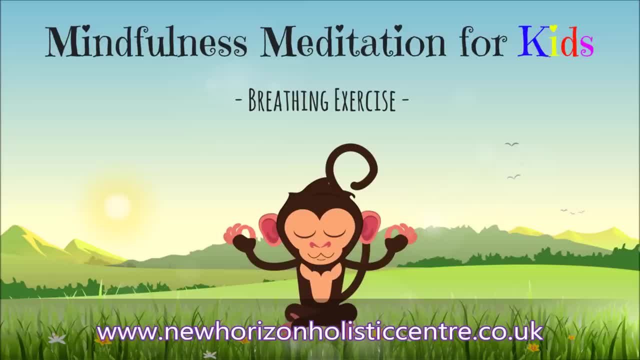 Good And breathe out slowly and gently One more time. deep breath in and breathe out slowly and gently, Keeping your eyes closed. notice the sounds around you. What can you hear? Feel the floor beneath your feet, Feel the chair you are sitting on. 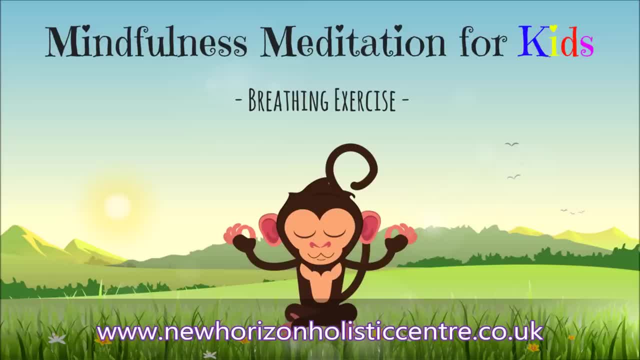 How does it feel? Does it feel soft or does it feel hard? Feel the clothes against your body. Now wriggle your fingers and wriggle your toes. Shrug your shoulders, stretch if you want to And whenever you are ready. 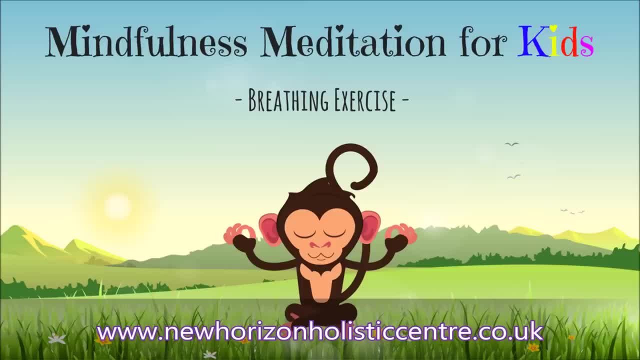 open your eyes, Breathe out slowly and gently. Keep your eyes closed and breathe in and breathe out gently and gently. Keep your eyes open and see if you get a sense of moving or moving. Keep your eyes closed and see if you get a sense of moving or moving. 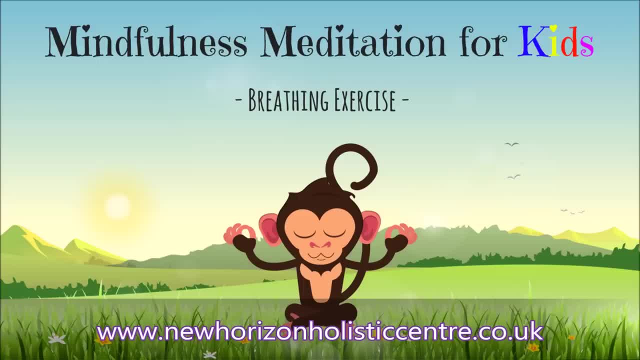 Do you feel it? No, you don't, No, you don't, You don't, You don't, No, you don't you.